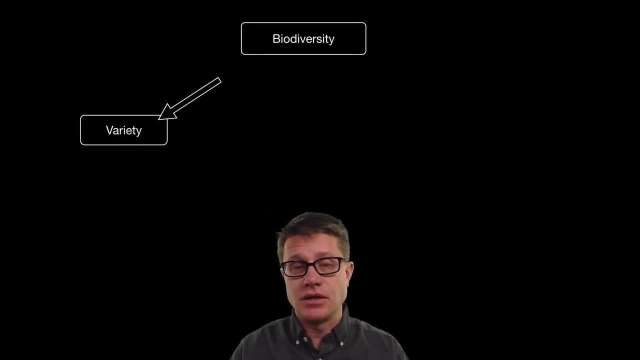 Lebanon, But it does kind of get at this idea of the importance of biodiversity. Biodiversity is not only species diversity, but it can be genes, It can be the species that are going to change Species, especially our domesticated crops and livestock, and then ecosystems themselves. 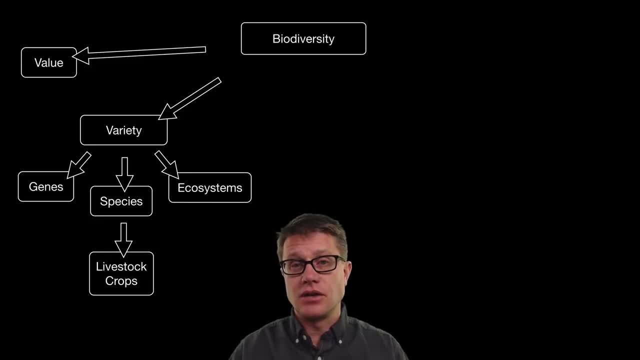 And they have value. They give us our resources and they also do these ecosystem services, And they are at risk. We are seeing biodiversity loss all around the planet. The causes are habitat loss, invasive species, climate change- We also have over harvesting- and then, finally, 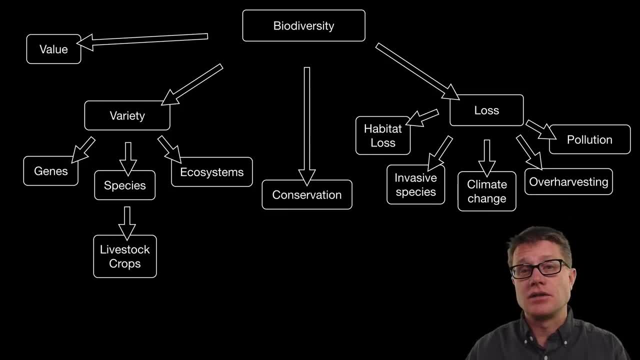 pollution are all impacting biodiversity, And so it has led to conservation. What do we do? first, We have to figure out where that biodiversity is being lost, We have to figure out the conservation status of these organisms or areas, And then, finally, we can pass laws. 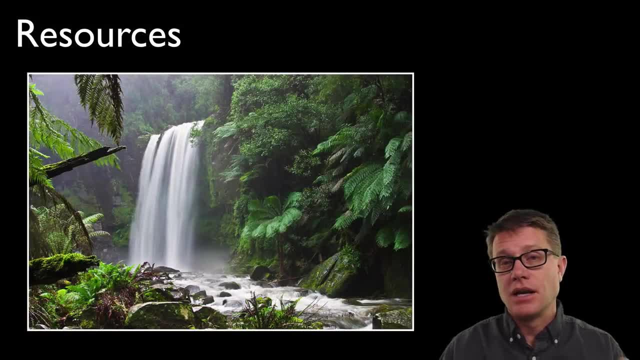 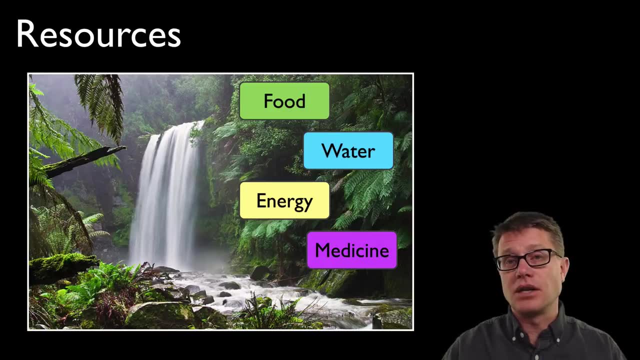 and treaties to try to preserve a lot of that biodiversity. And so again, why do we need biodiversity? It is where we get our food, It is how we filter our water, energy, medicine- We all get that from our environment. And again, our environment also does these ecosystem. 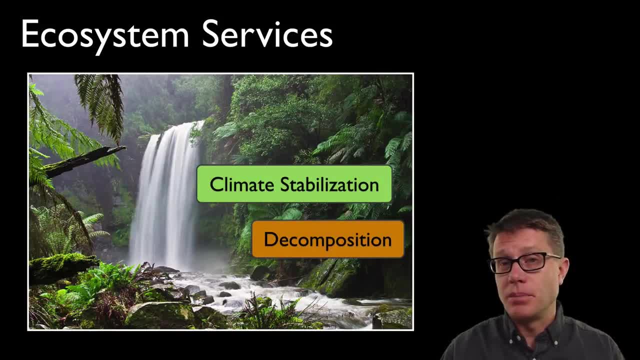 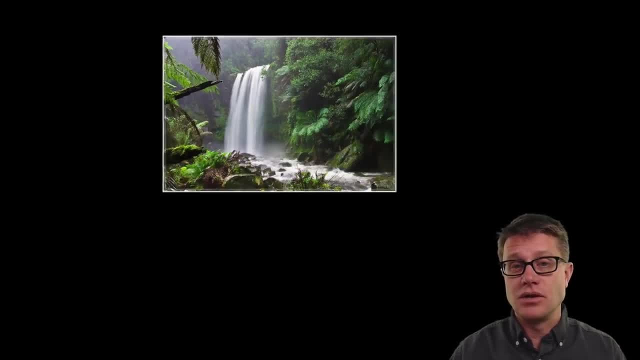 services. They keep our climate stable, They decompose material once it has died, They pollinate our crops, And so we need biodiversity on our planet for resources and to do the services. If we define what it is, it is simply variety, Variety at the genetic level. 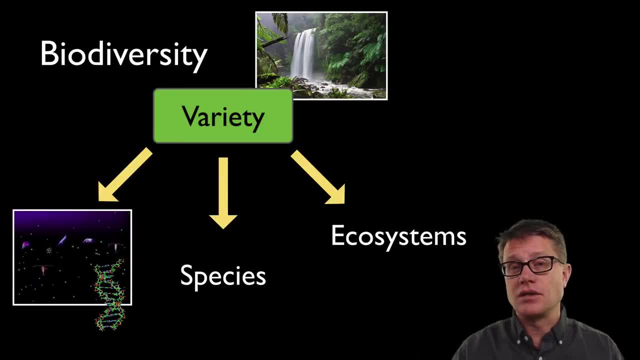 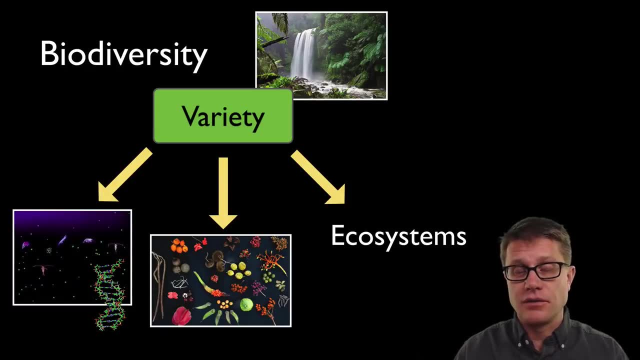 at the species level and at the ecosystems, And so those genes that organisms have. once the organism is gone, or the gene is gone, it is gone forever. It is extinct Species as well. These are all the fruits found in a certain area of the tropical rainforest. 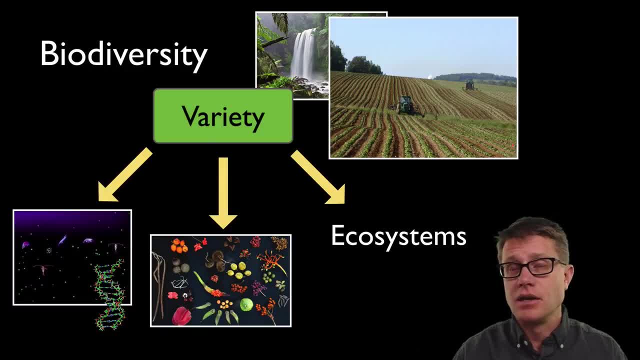 But also we are talking about the crops that we have, And so I think it used to be. we had around 8000 different types of apples that were being grown, And now it is 100. And if you look in your own supermarkets, you can see that there are a lot of different types. 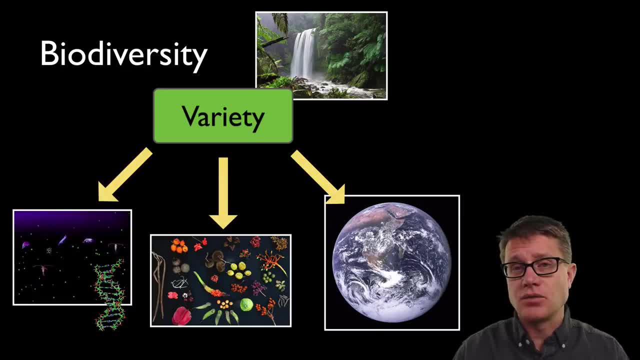 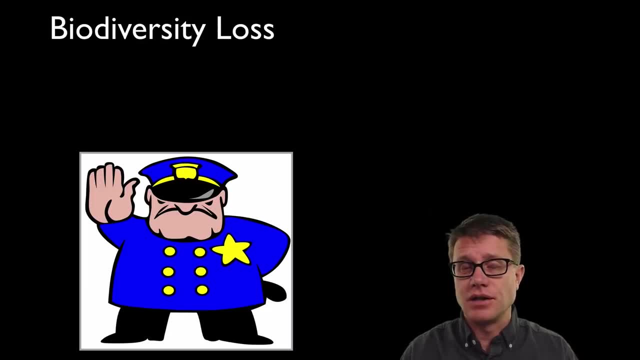 of apples. And then it is ecosystem changes as well. Once an ecosystem is gone- coral reefs, for example- you cannot build that back again. And so what is causing this biodiversity loss? Well, when I was trying to come up with a quick way for you to remember these five, 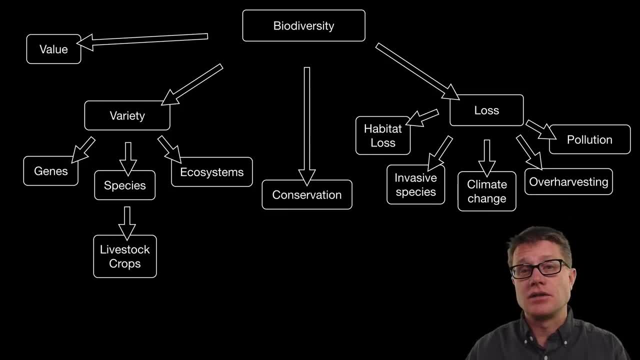 pollution are all impacting biodiversity, And so it has led to conservation. What do we do? first, We have to figure out where that biodiversity is being lost, We have to figure out the conservation status of these organisms or areas, And then, finally, we can pass laws. 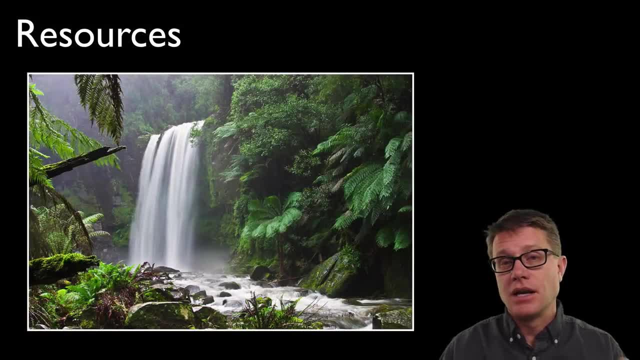 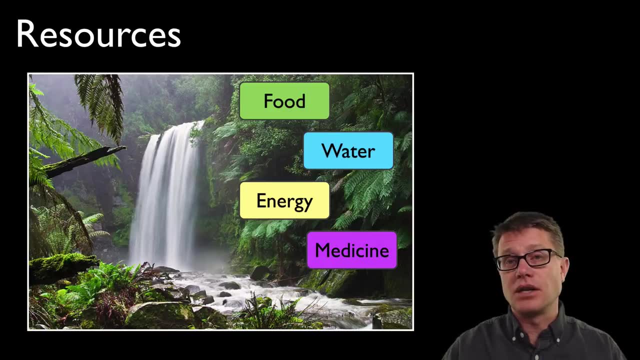 and treaties to try to preserve a lot of that biodiversity. And so again, why do we need biodiversity? It is where we get our food, It is how we filter our water, energy, medicine- We all get that from our environment. And again, our environment also does these ecosystem. 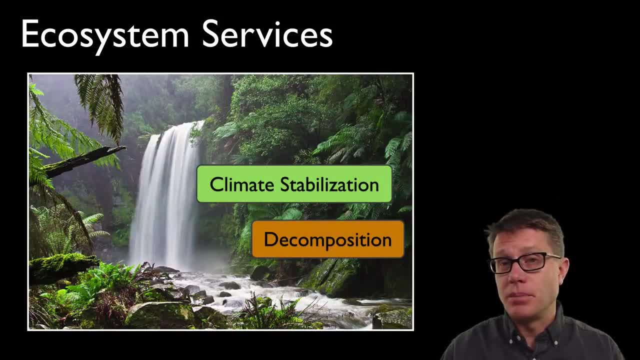 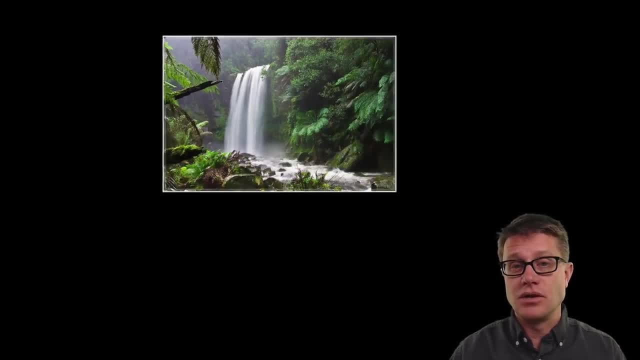 services. They keep our climate stable, They decompose material once it has died, They pollinate our crops, And so we need biodiversity on our planet for resources, and to do that, We do these services. If we define what it is, it is simply variety, Variety at the 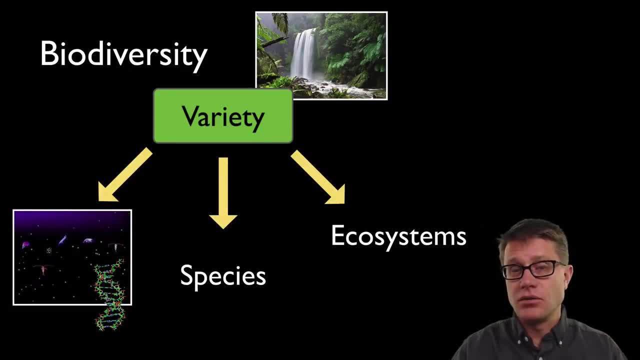 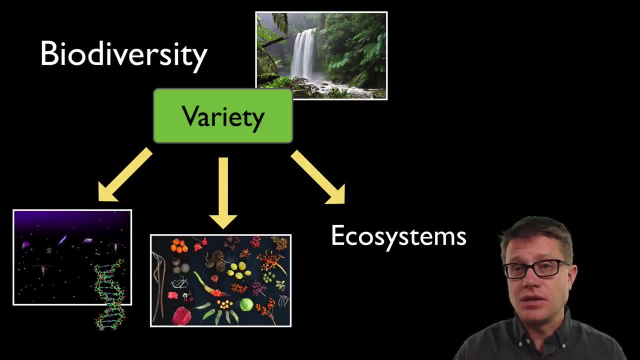 genetic level, at the species level and at the ecosystems, And so those genes that organisms have. once the organism is gone, or the gene is gone, it is gone forever. It is extinct Species as well. These are all the fruits found in a certain area of the tropical rainforest. 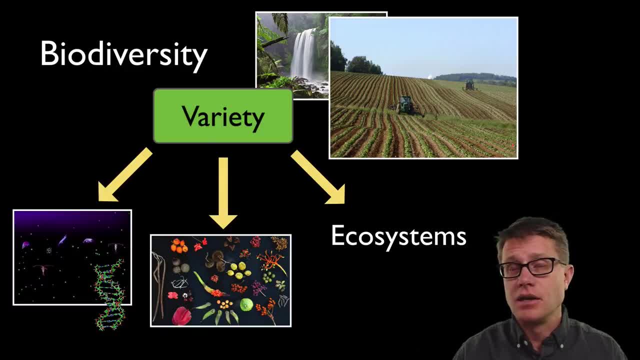 But also we are talking about the crops that we have, And so I think it used to be. we had around 8000 different types of apples that were being grown, And now it is 100. And if you look in your own supermarkets, you can see that there are a lot of different types. 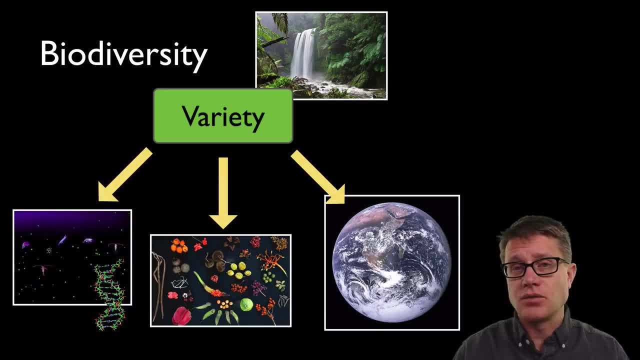 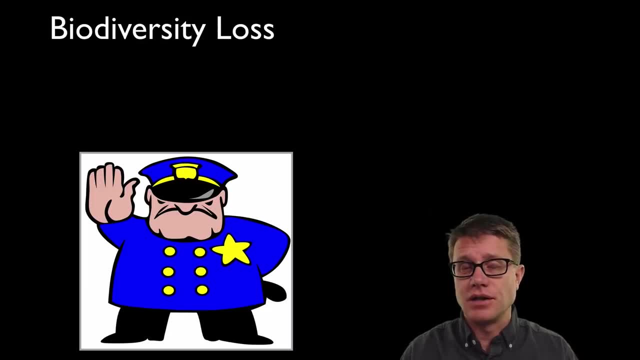 of apples, And if you look in your own supermarket, it is way less than that. And then it is ecosystem changes as well. Once an ecosystem is gone- coral reefs, for example- you cannot build that back again. And so what is causing this biodiversity loss? Well, when I was trying, 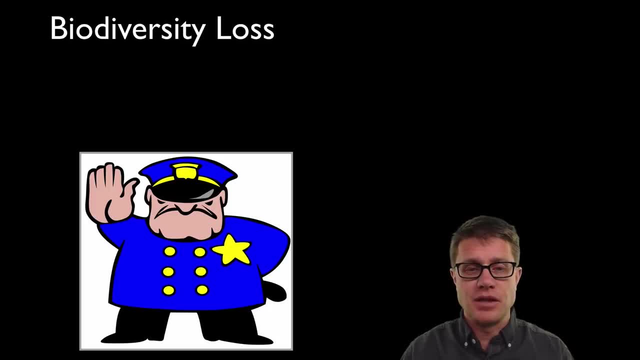 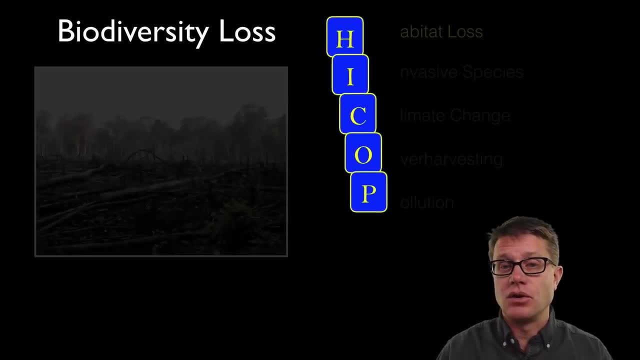 to come up with a quick way for you to remember these five things. I came up with this mnemonic And so, if you think of the biodiversity cop and if you think of high cop as a way to remember it, if we put those in order, habitat loss is the first big impact on biodiversity. So 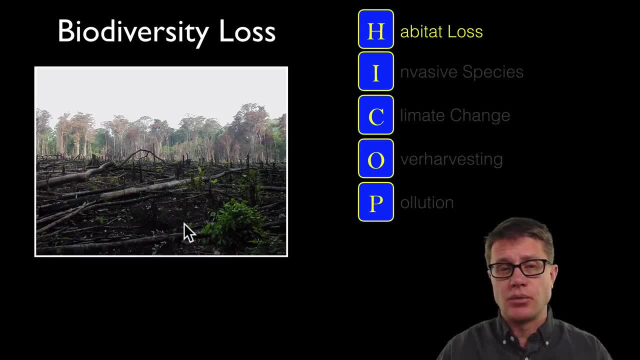 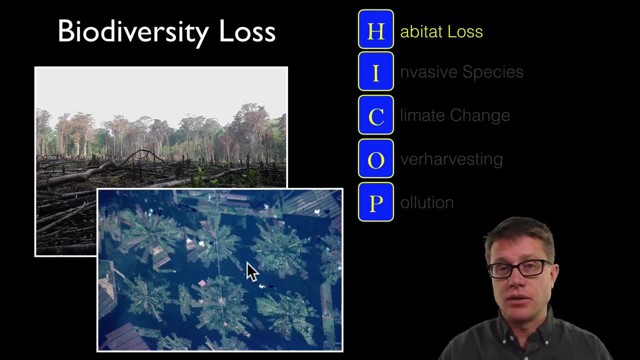 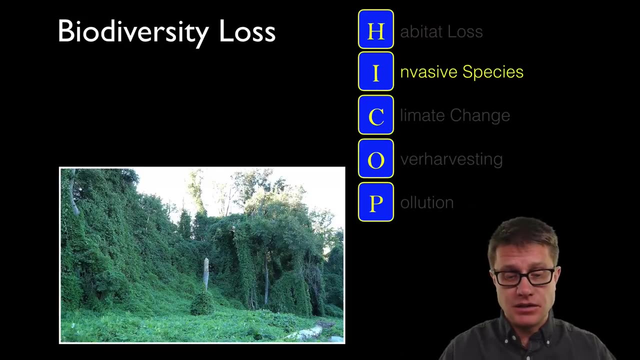 deforestation when we are cutting down. By that we are showing back down into those rainforests and planting crops. Right here we are growing soybeans. This is looking from above, where we used to have a tropical rainforest. We are reducing that diversity and we are replacing it with one simple crop: Invasive. 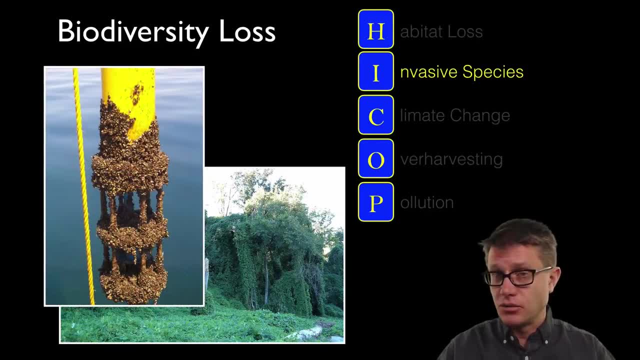 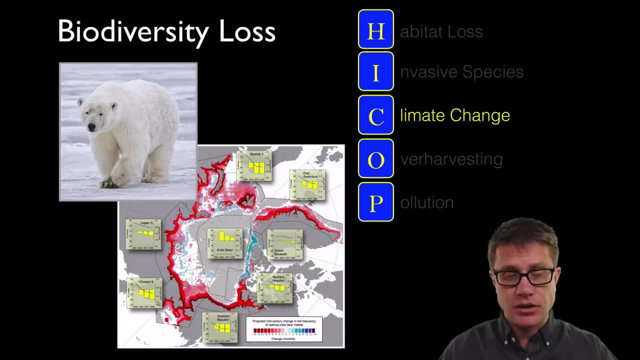 species. this is Kudzu. This is a plant that was brought from Asia. These are the zebra mussels in the Great Lakes that are really winking havoc. They came from the Mediterranean. We are also seeing climate change impacting biodiversity. So if we look at a polar bear, 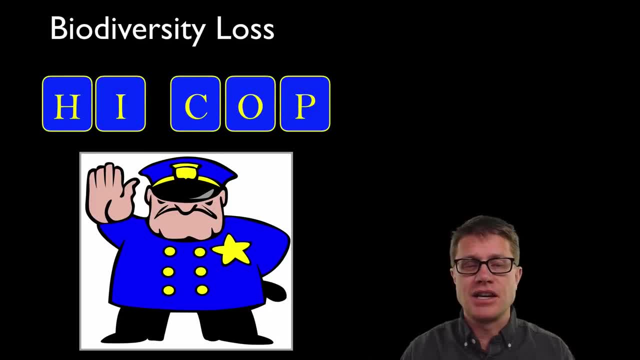 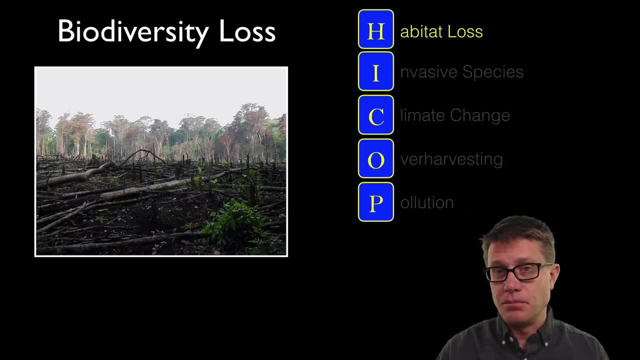 things. I came up with this mnemonic And so if you think of the biodiversity cop and if you think of high cop as a way to remember it, if we put those in order, habitat loss is the first big impact on biodiversity. So deforestation- when we are cutting down, we 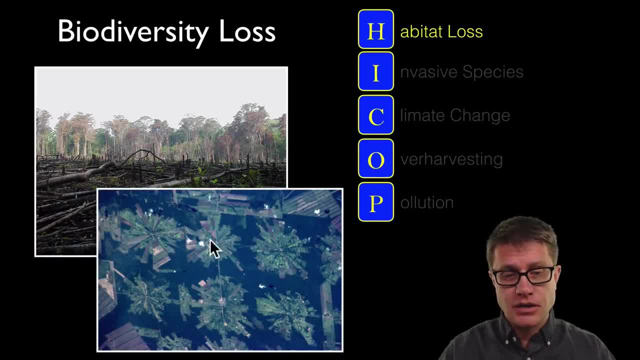 are cutting down those rainforests and planting crops. Right here we are growing soybeans. This is looking from above, where we used to have a tropical rainforest. We are reducing that diversity and we are replacing it with one simple crop- Invasive species. This is. 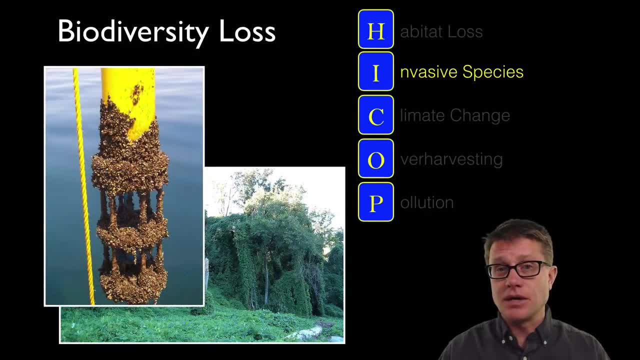 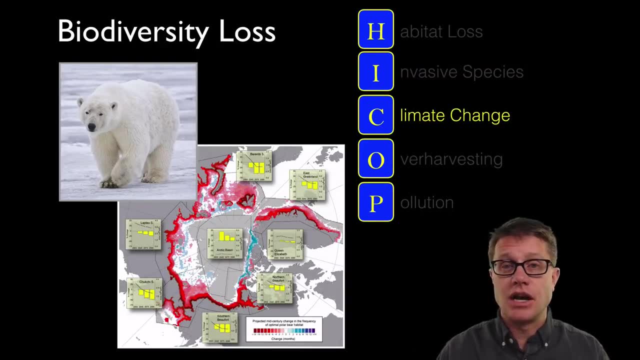 kudzu. It is a plant that was brought from Asia. These are the zebra mussels in the Great Lakes that are really wreaking havoc. They came from the Mediterranean. We are also seeing climate change impacting biodiversity. So if we look at the polar bear, for example, 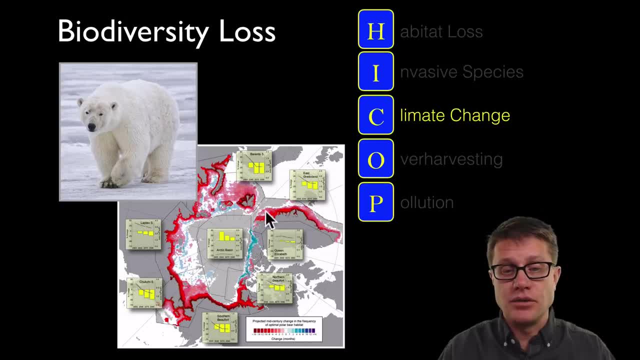 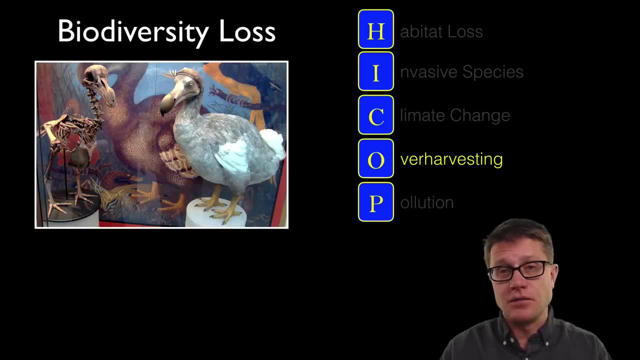 will they go extinct? It is hard to tell, But if we look at all the areas where they used to do well, we are seeing a decrease in the optimal polar bear habitat. Also, over harvesting: Humans have been harvesting animals for a long period of time. The dodo is extinct. 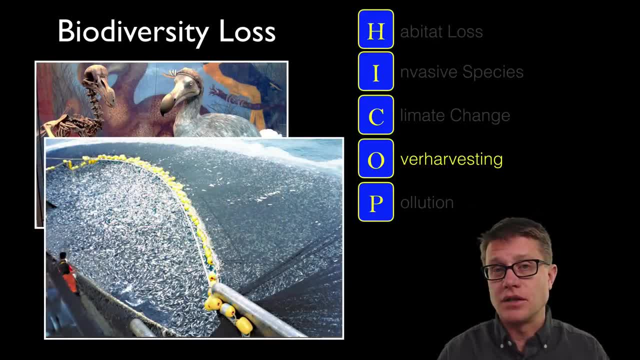 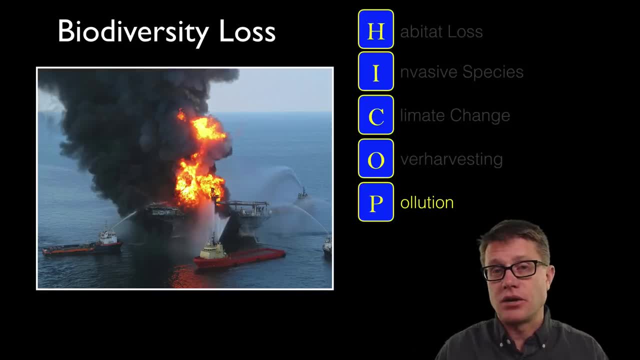 because we killed all of the dodos And we are also seeing over harvesting now, especially in our aquatic systems, And then we can have pollution. Pollution is impacting the environment as well. So if we look at that deep water horizon explosion that led to an oil spill, 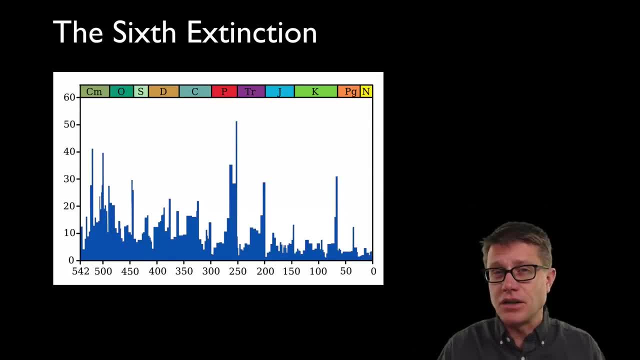 which is impacting biodiversity in the Gulf of Mexico. And then we have a lot of other things happening in the Gulf of Mexico, And it will take us years to figure out how that impacts it. Now this has been going on for a long period of time. Extinctions are a part. 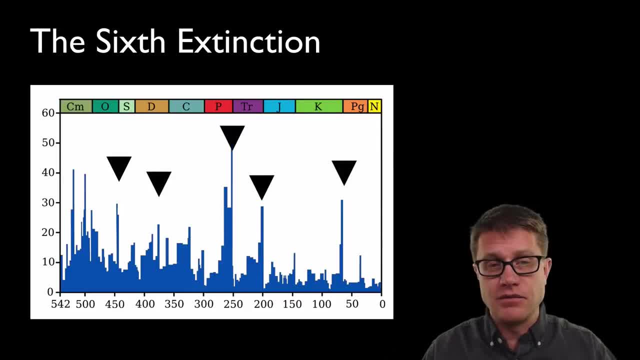 of nature And if we look back through the fossil record, we have seen five major mass extinctions over time And they have different causes, But most scientists are pointing to right now as the sixth mass extinction. This is mass extinction caused by humans. We are 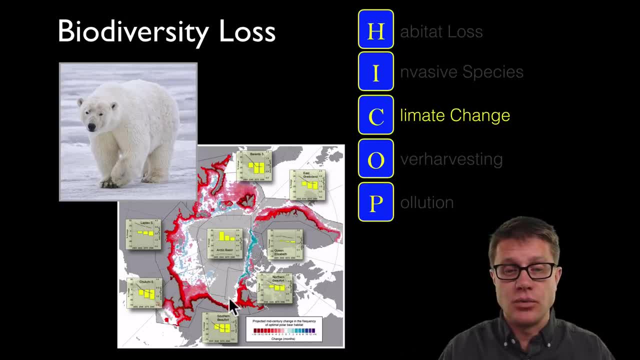 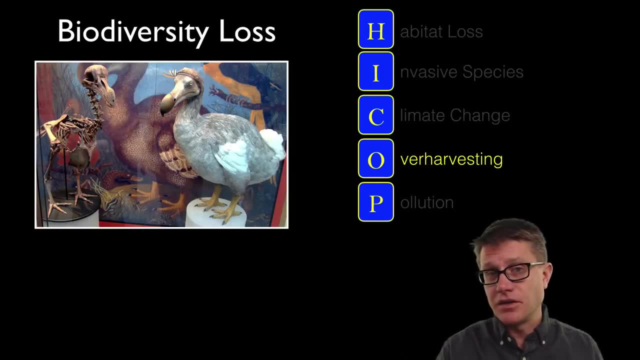 extinct. It is hard to tell, But if we look at all the areas where they used to do well, we are seeing a decrease in the optimal polar bear habitat. Also, over harvesting Humans have been harvesting animals for a long period of time. The dodo is extinct because we killed 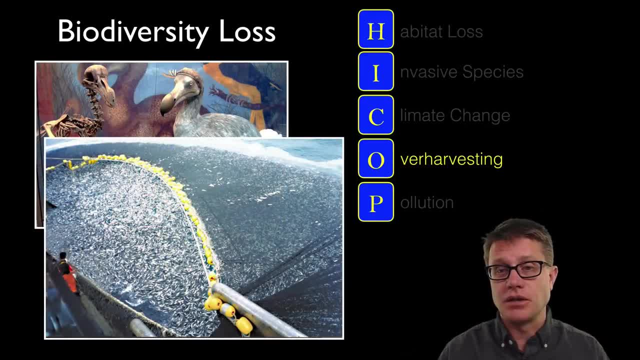 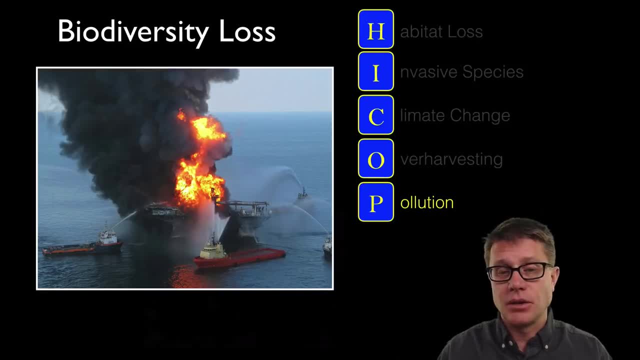 all of the dodos And we are also seeing over harvesting now, especially in our aquatic systems, And then we can have pollution. Pollution is impacting the environment as well. So if we look at that deep water horizon explosion that led to an oil spill, which is impacting- 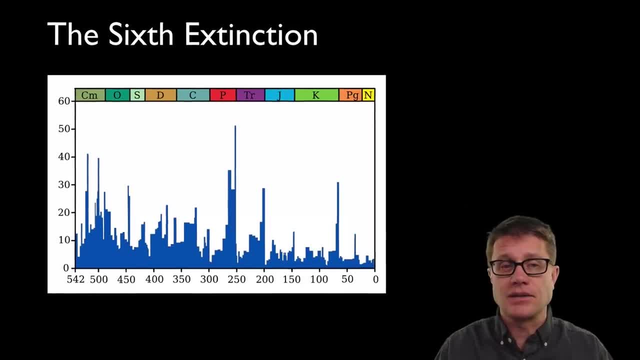 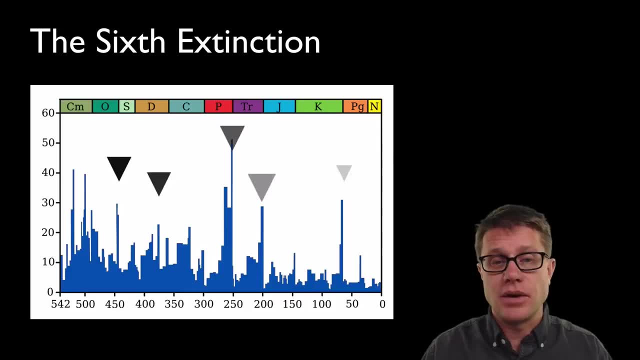 biodiversity in the Gulf of Mexico, And it will take us years to figure out how that impacts it. Now, this has been going on for a long period of time. Extinctions are a part of nature And if we look back through the fossil record, we have seen five major mass. 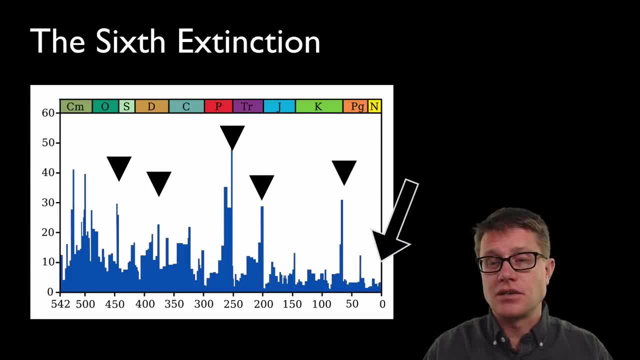 extinctions over time And they have different causes, But most scientists are pointing to right now as the sixth mass extinction. This is mass extinction caused by humans. We are seeing extinction rates that we have never seen before Biodiversity loss that we have. 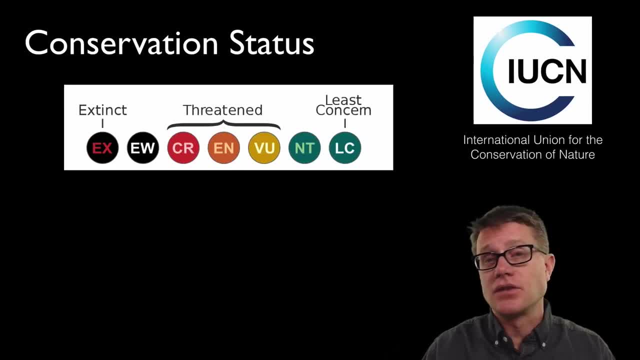 never seen before, And its cause is us. And so how do we solve this problem? Well, the first step is to identify where the problem is, And so the IUCN- International Union for the Conservation of Nature- has been around for over half a century, And what they have done is come up with these different statuses. 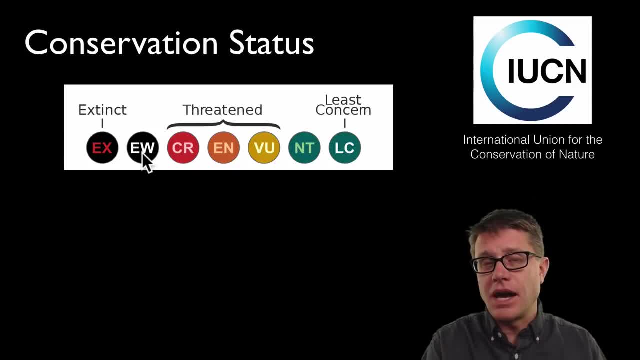 Extinct. Extinct in the wild would be one where we maybe have them in a zoo, but they do not exist in the wild. Then we have critically endangered, endangered and vulnerable. Then we have near threatened and finally, areas of least concern. And so, if you go on Wikipedia, 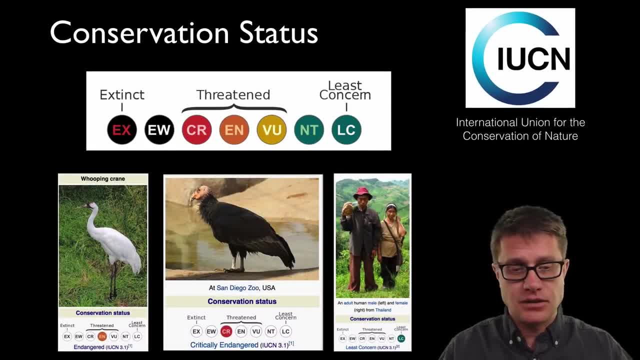 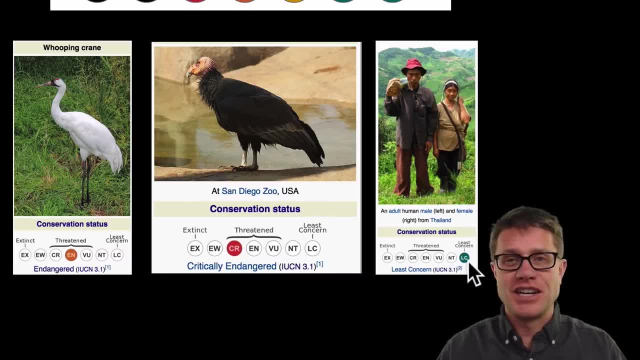 you can look up any animal or any plant and it is going to tell you its conservation status. So, for example, the whooping cranes are endangered. The California condor is critically endangered. Humans, you can imagine, are an area of least concern. They have then created. 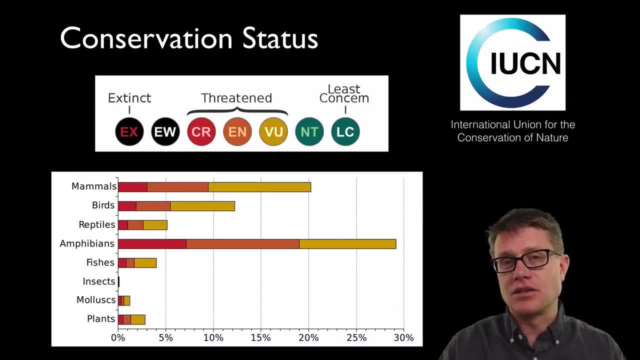 this red list where we look at how many of these species fall into these threatened or these red categories. If we look at mammals, almost 20% or over 20% are in this threatened kind of an area, And amphibians are really at risk. And so what do we do? Well, what we 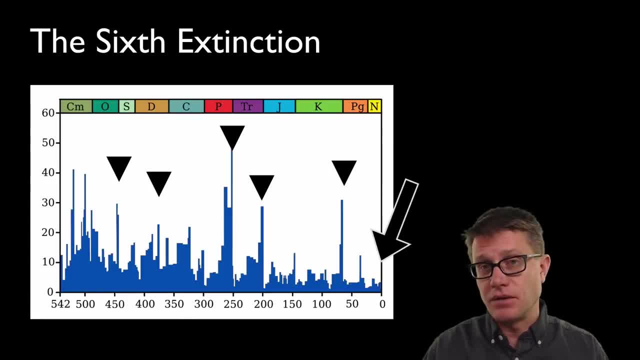 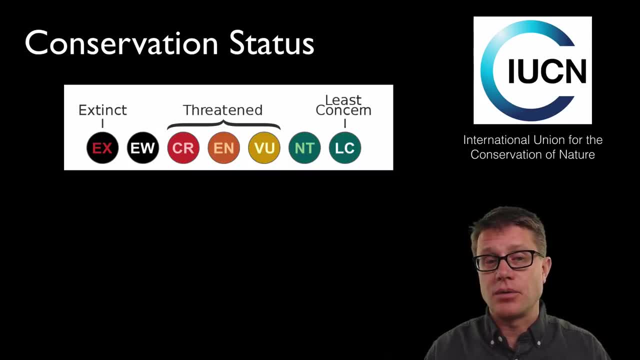 seeing extinction rates that we have never seen before, Biodiversity loss that we have never seen before, And its cause is us. So how do we solve this problem? Well, the first step is to identify where the problem is, And so the IUCN- International Union for the Conservation of Nature- has been around. 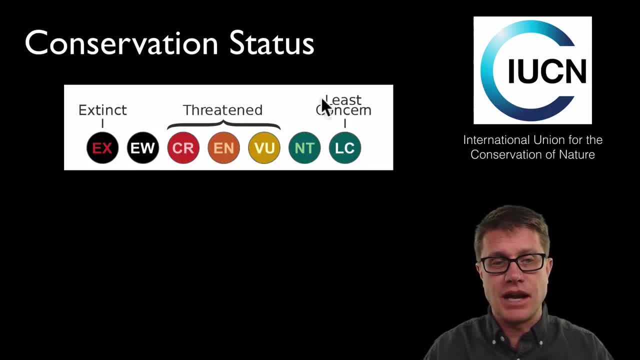 for over half a century, And what they have done is come up with these different statuses. Extinct in the wild would be one where we maybe have them in a zoo, but they do not exist in the wild. Then we have critically endangered- endangered and vulnerable. Then we have near. 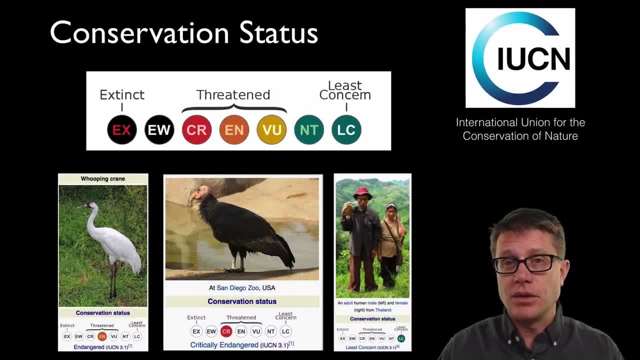 threatened and, finally, areas of least concern. And so if you go on Wikipedia, you can look up any animal that is endangered and vulnerable, And then you can look up any animal that is a pet animal or any plant that is going to tell you its conservation status. So for, 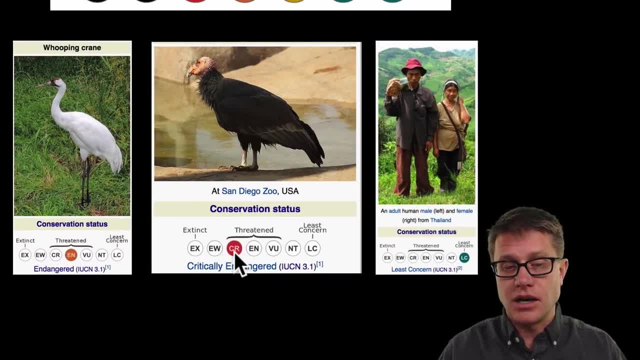 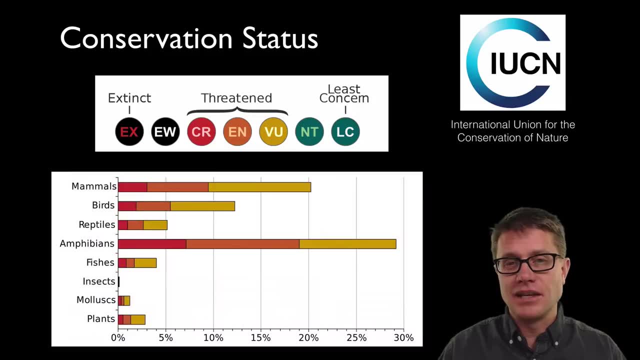 example, the whooping cranes are endangered. The California Condor is critically endangered. Humans, you can imagine, are in the area of least concern. They have then created this red list where we look at how many of these species fall into these threatened or these. 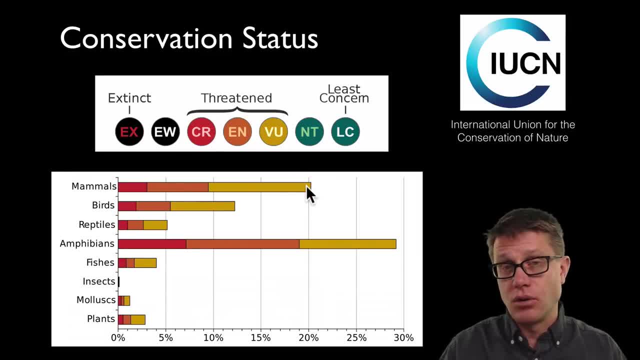 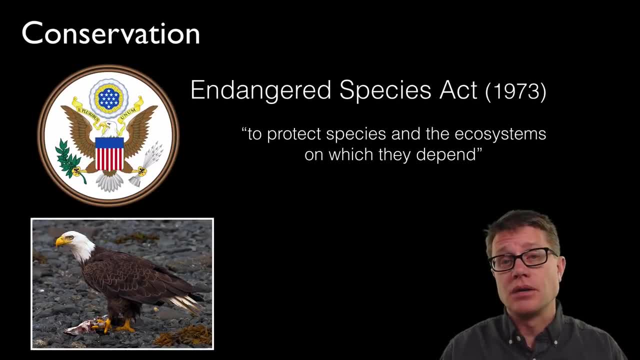 red categories. If we look at mammals, almost 20% or over 20% are in this threatened kind of an area, And amphibians are really at risk. And so what do we do? Well, what we can do is pass laws us. we passed the Endangered Species Act in 1973 to protect species and the ecosystems. 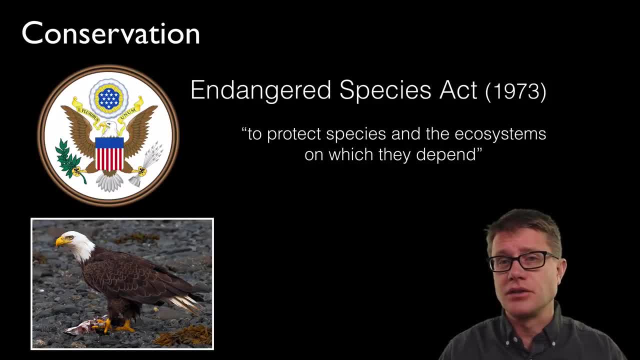 on which they depend, And so it essentially is a list. So bald eagles are a classic example that were added to the endangered species list, And so there, I think, were around 500 breeding pairs in the lower 48. And now there is over 10,000.. So once they recover, we remove. 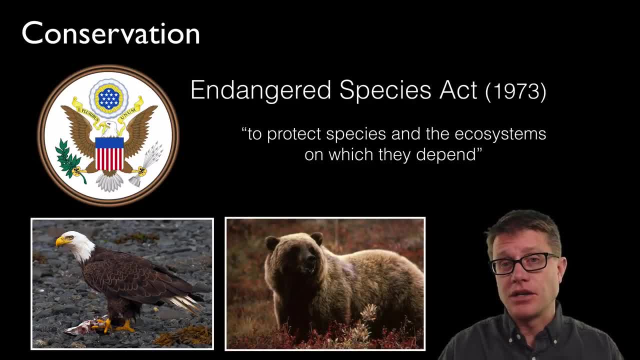 them from that list. Grizzly bears were added. Their population is coming back In Montana. there is a big debate right now over do we remove them from the list or not. But it also has to be balanced with human resources as well, So logging, for example, can impact. 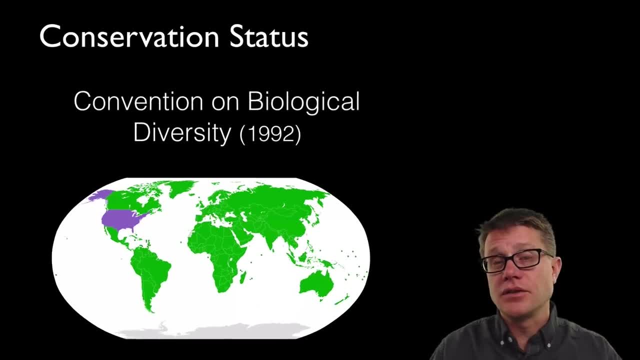 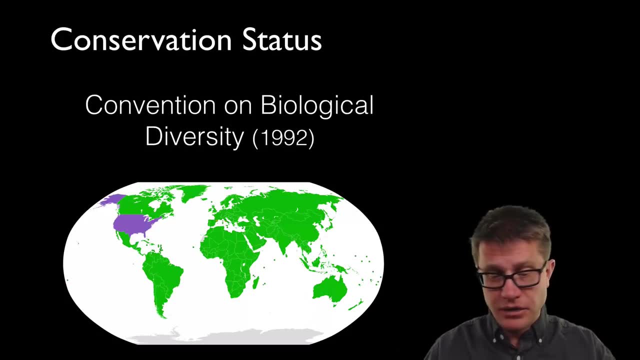 certain species that are going to be found on the endangered species list. We have also seen global changes: The Convention on Biological Diversity in 1992.. All of the green countries here signed on that. biodiversity is important, It has an economic import And that we are. 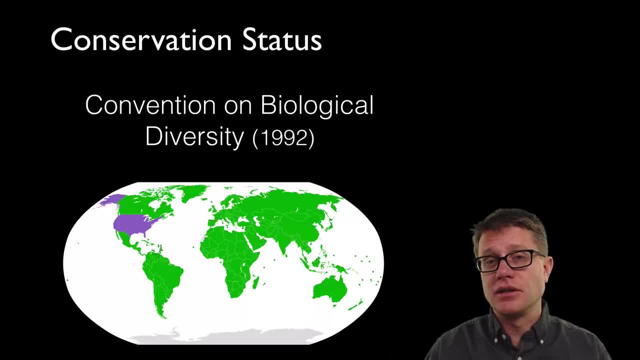 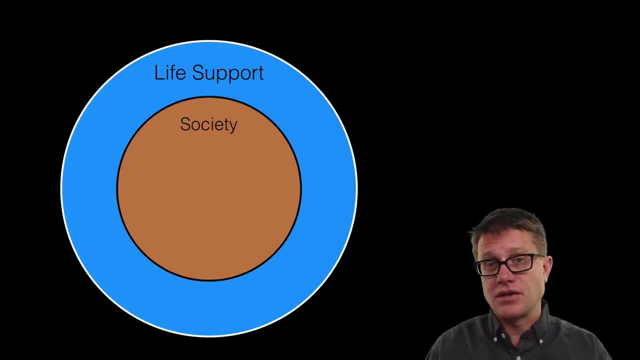 going to try to protect it, But again, it is not legally binding, And so we are still seeing huge, deep changes, Decreases in biodiversity, And it goes back to the first thing I talked about in this class: The idea that the planet supports society, but society is driven by economics, And so 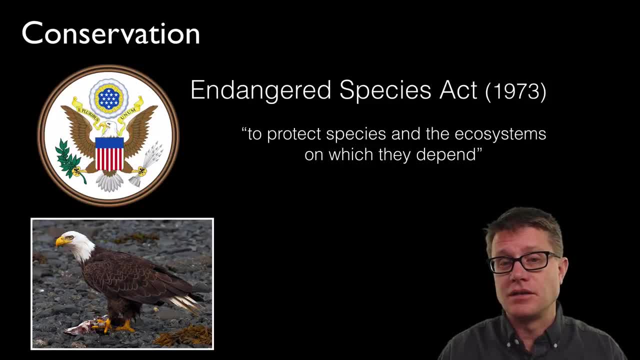 can do is pass laws. So what we can do is pass laws. So what we can do is pass laws. So in the US, we passed the Endangered Species Act in 1973 to protect species and the ecosystems on which they depend, And so it essentially is a list. So bald eagles are a classic example. 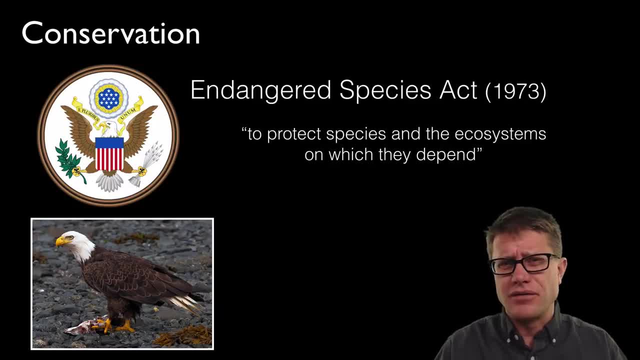 that were added to the endangered species list, And so there, I think, were around 500 breeding pairs in the lower 48. And now there is over 10,000. So once they recover we remove them from that list. Grizzly bears were added. Their population is coming back In Montana. 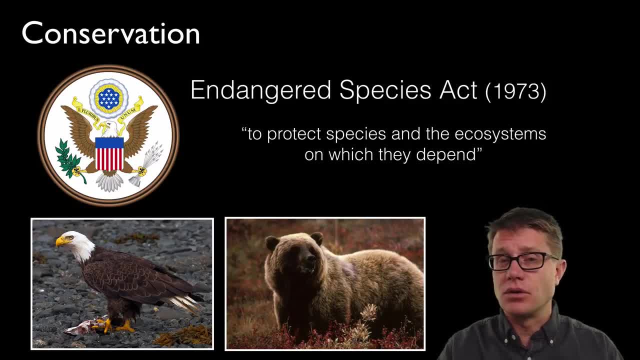 there is a big debate right now over do we remove them from the list or not, And so we can do that, But it also has to be balanced with human resources as well. So logging, for example, can impact certain species that are going to be found on the endangered species. 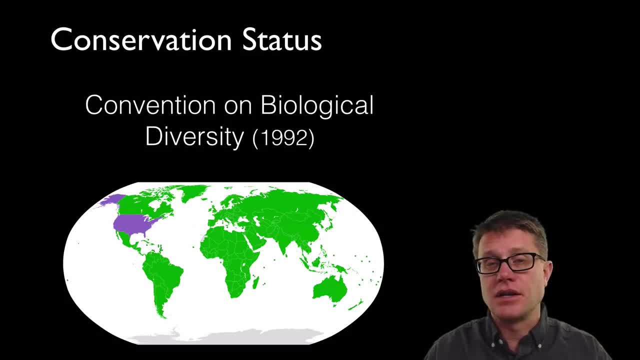 list. We have also seen global changes: The Convention on Biological Diversity in 1992.. All of the green countries here signed on that biodiversity is important, It has an economic import And that we are going to try to protect it. But again, it is not legally. 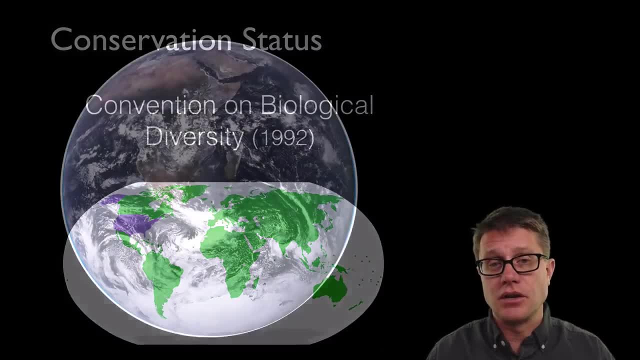 binding, And so we are still seeing huge decreases in biodiversity. And it goes back to the first thing I talked about in this class, The idea that we are going to try to protect it. But again, it is not legally binding, And so we are still seeing huge decreases in biodiversity. 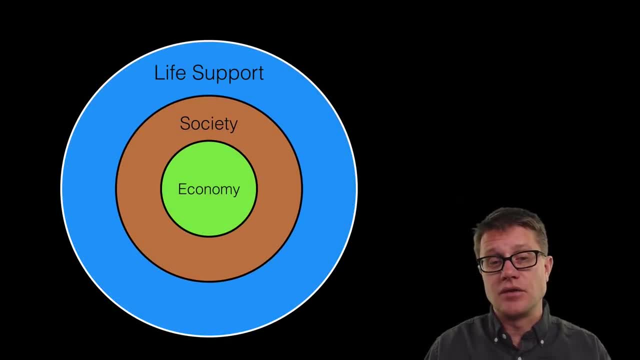 And it goes back to the first thing I talked about in this class: The idea that we are going. the planet supports society, But society is driven by economics, And so we are never going to see decreases in biodiversity loss until there is an economic incentive or a 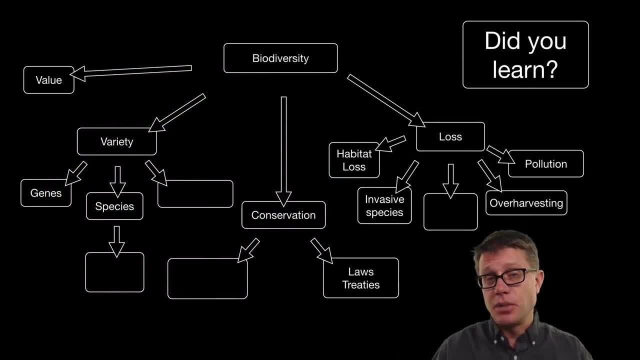 way to do that, And so did you learn the following. Could you pause the video at this point and fill in the blanks? Well, let me do that for you. Biodiversity has value. It is a variety in the genes, species and eco-systems- Again, especially the domestic ones- that we 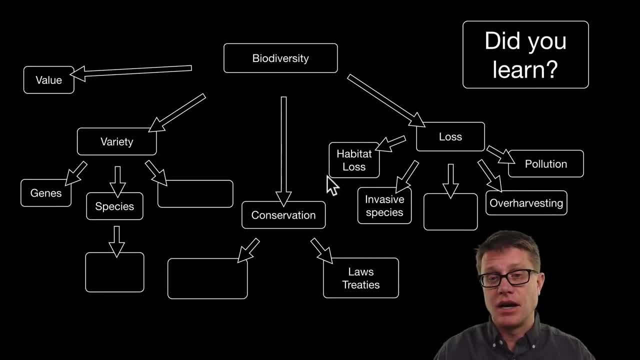 need to survive. That loss is caused by high COP. So that is habitat loss, invasive species, species, climate change over harvesting and pollution. And then how do we solve this? Through conservation, we figure out the status of those organisms, or maybe those ecosystems. 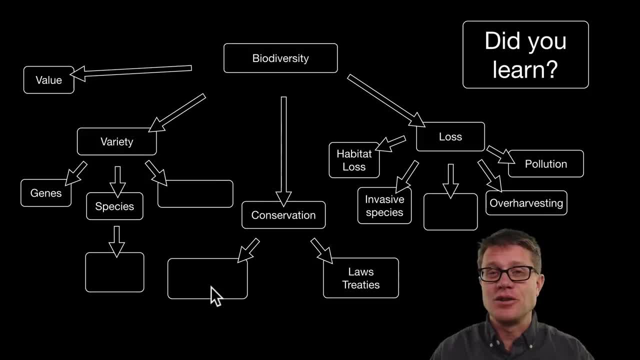 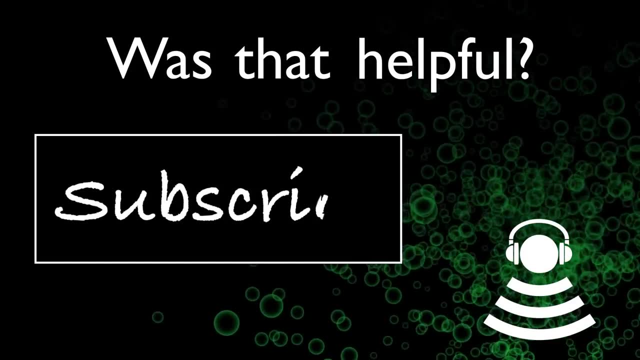 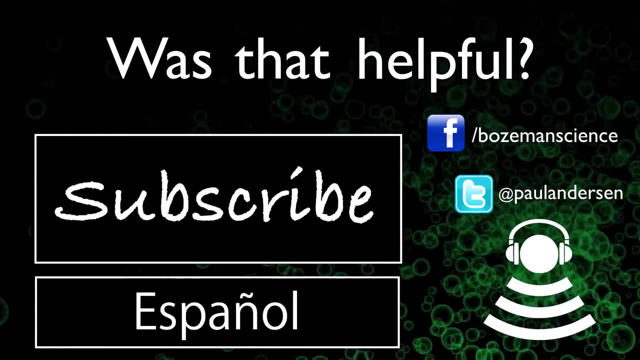 And then we start to protect them through laws and treaties. So that is it, And it is also the last of the videos on AP Environmental Sciences, So I hope that was helpful. Subtitles by the Amaraorg community.